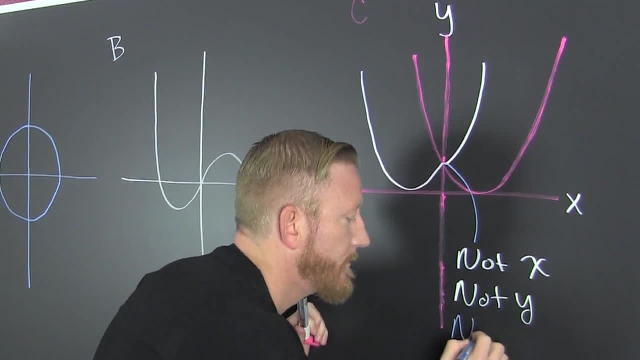 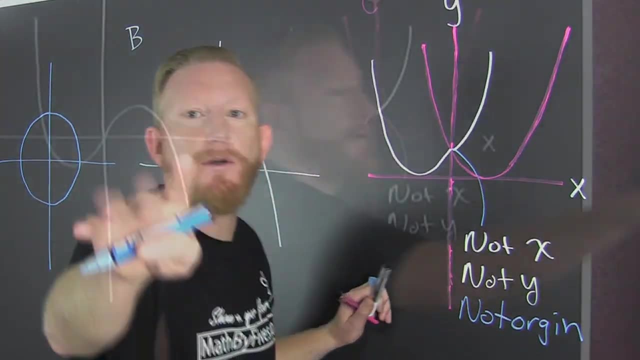 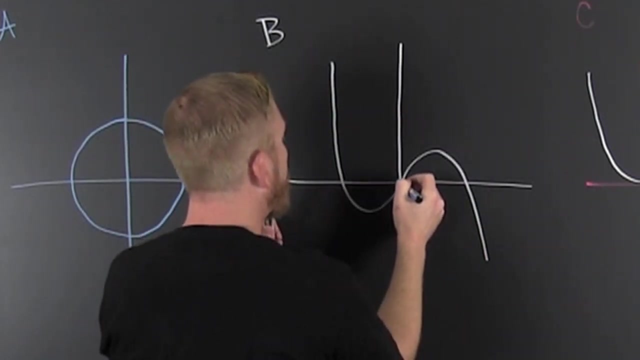 Bam. It doesn't lie on itself, so it's not origin. Is that how I spell origin? I don't even know Whoa Over here. to this middle example: if I flip it on the x boom, then no, it doesn't lay on itself, so it's not. 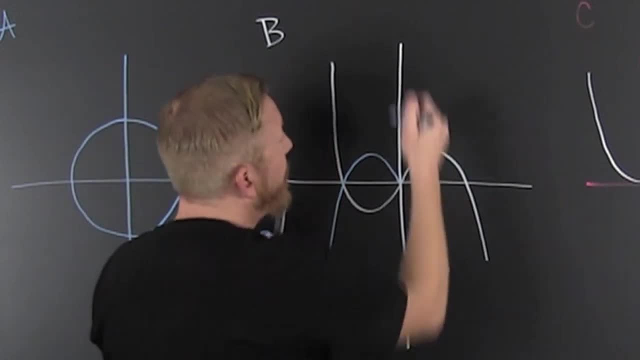 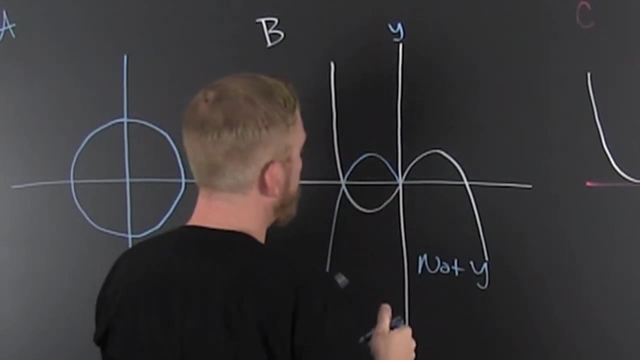 x. Pardon, this is y, It's not y. If I were to flip it on the x, then it's a bam and bam It's not x. But if I flip it on, if I flip it about y, 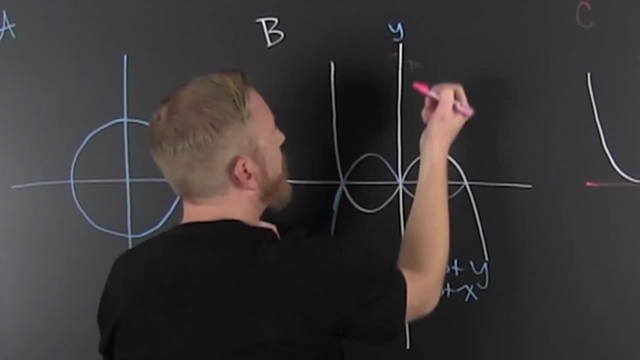 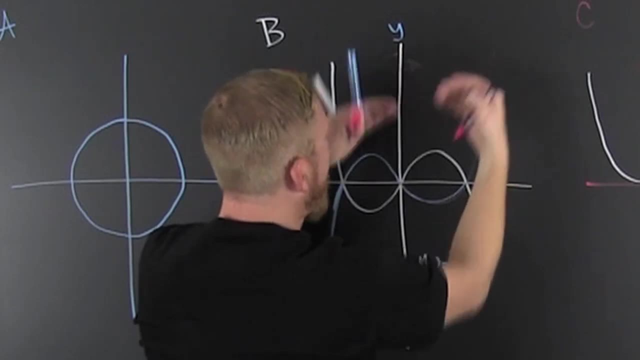 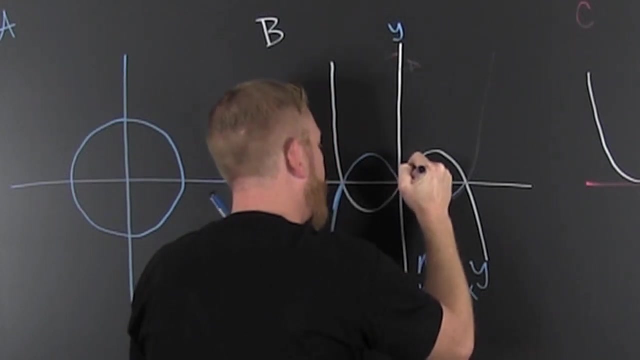 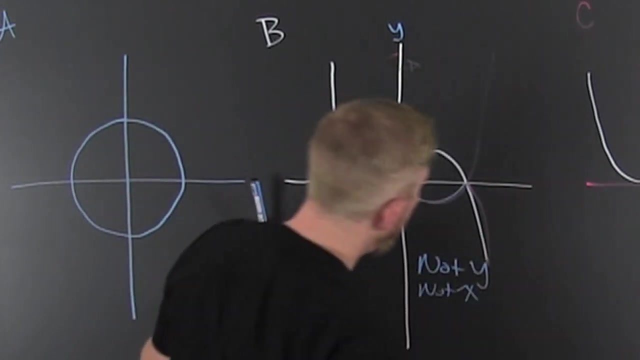 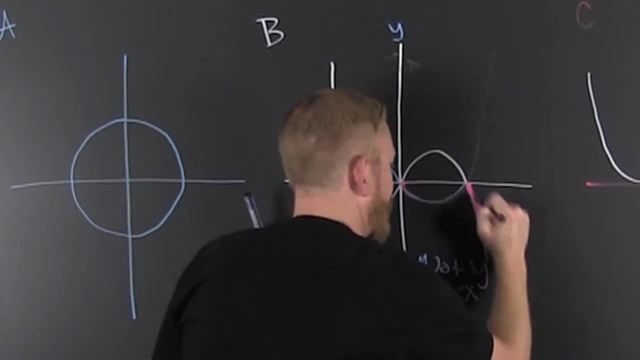 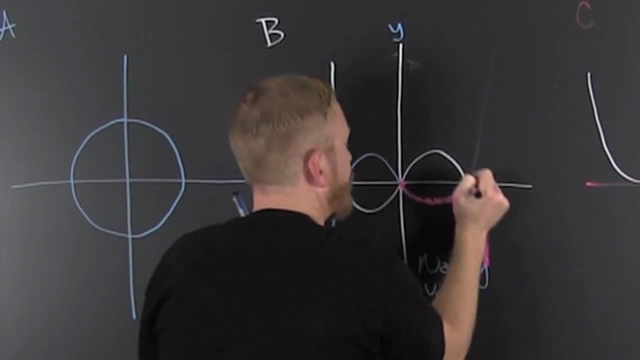 Come on pink, We're going to get you to work. It's five bucks a piece, Yeah, So what I do? I first flipped on y bam and then I flipped on x bam and it lays on top of itself. So this is origin. 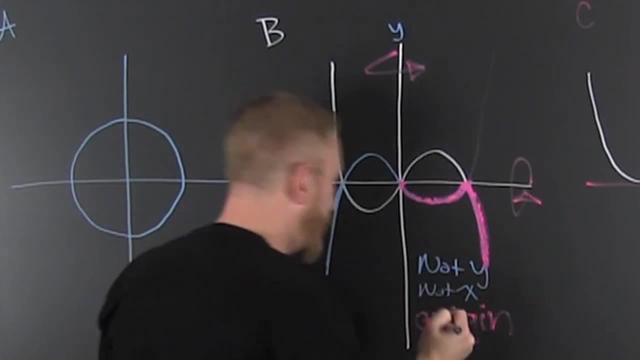 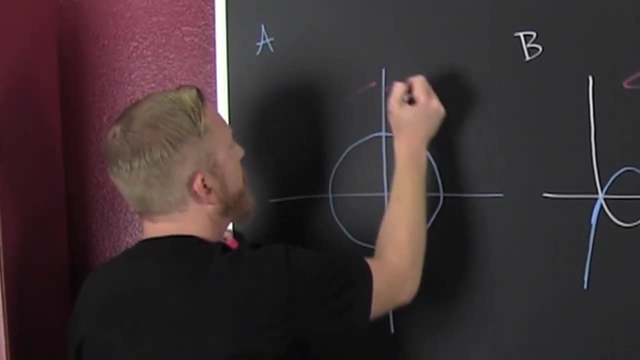 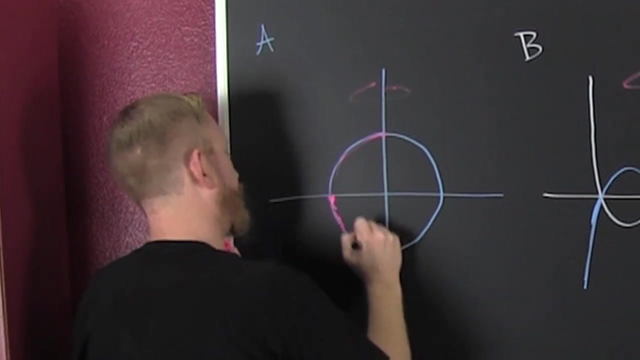 Origin. I don't know. Come on pink, You're going to pull through this. Let's do this one over here. Oh, so if I flip it across the y-axis, if I flip it across the y-axis, ah, so it's y-symmetry. 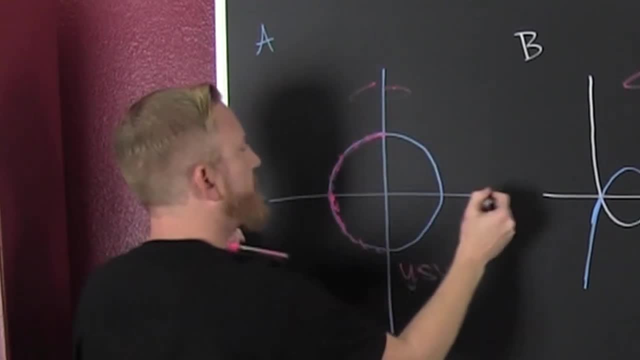 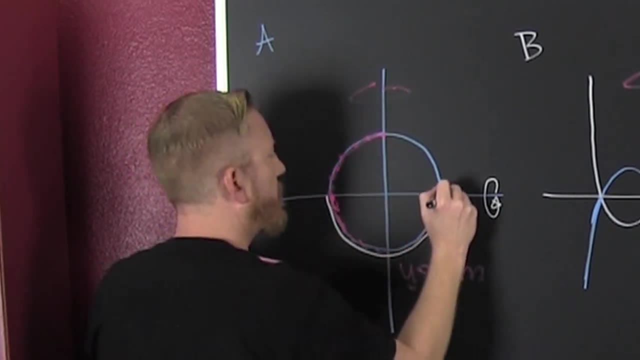 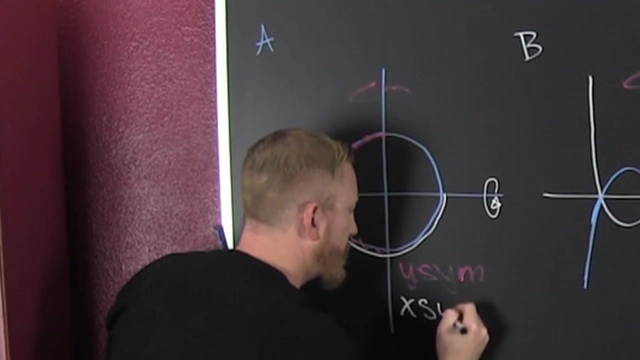 Ah, what if I flipped it across the x? If I flipped it across the x, Oh, you're working fine. So, hmm, I didn't want to get my colors mixed up. If I flip it across the x, it lays on itself, So it's x Symmetric.